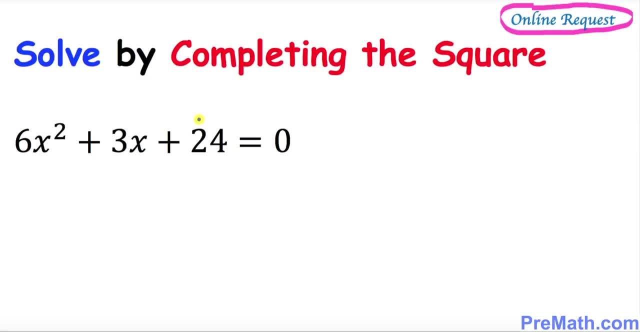 Hello again everyone. In this video tutorial we are going to solve this given quadratic equation by completing the square method. So the very first step is: we want to make sure that our leading coefficient must be 1.. In our case, our leading coefficient is 6.. We want to make it 1,. 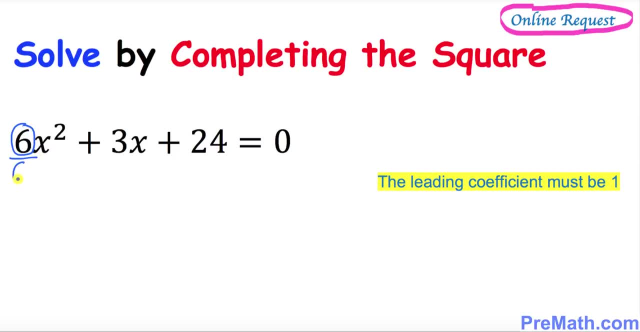 so we are going to divide this one by 6.. If you divide this one by 6, you must divide each and every term across the board by 6.. So let's go ahead and simplify. 6 over 6 simply becomes 1x squared plus. this 3 over 6 could be written as 1 over 2. 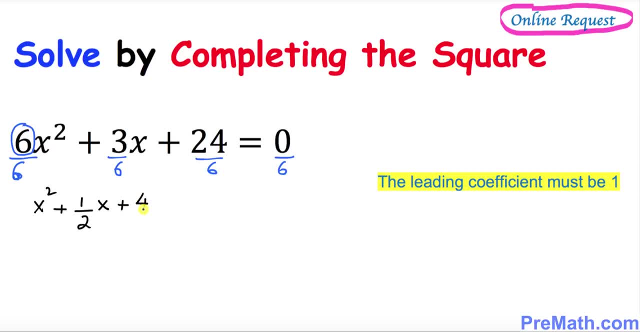 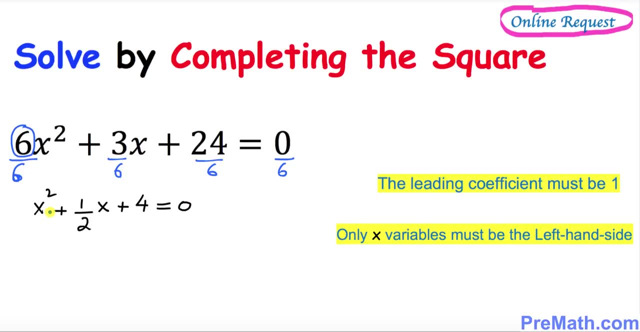 x plus 4 equal to 0.. In our next step we want to make sure that only x variable must be on the left hand side. That means this number 4 must go on the right hand side. So we can write this as: 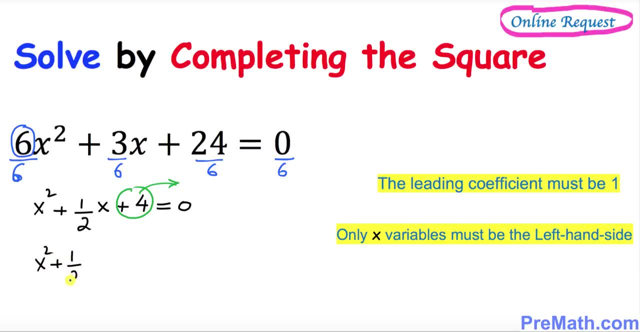 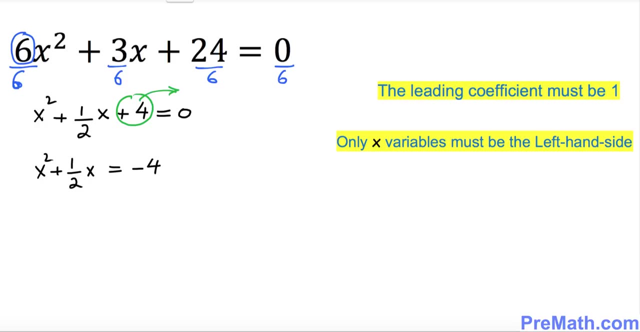 x squared plus 1 over 2 x equals 2.. You move this positive 4 on the other side becomes negative 4.. So far, so good. So now we're going to take care of this thing. I want you to just simply focus on this part over here. the coefficient of x. 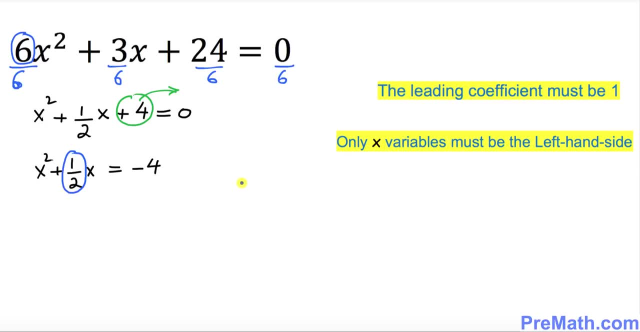 Don't worry about this sign. You put down this coefficient of x, which is 1 over 2, right up here. I want you to divide this number by this number. I want you to divide this number by this number. I want you to divide this number by this number. 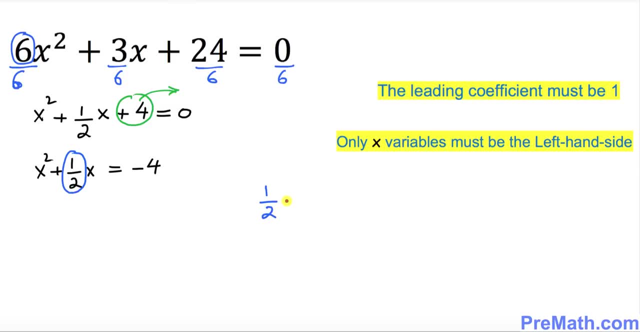 By 2.. Dividing by 2 is same as multiplying by 1 over 2.. Once you multiply this thing, 1 times 1 is 1 over, 2 times 2 is 4.. So always the very first step is you multiply by 1 over 2.. 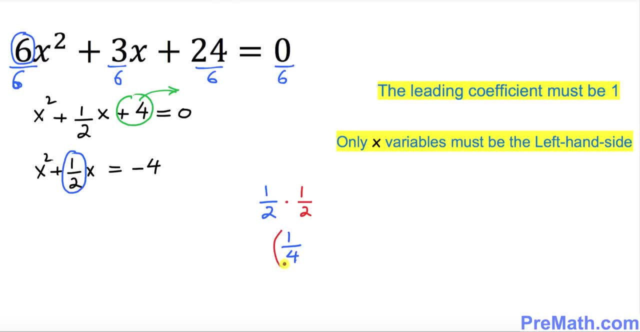 And then the next step is: whatever quantity you got, you must always square it. So we're gonna add this quantity, whatever this quantity, on both sides of these equation. Let's go ahead and put it down, that one, so we can write down: x squared plus 1 over 2, x plus equals. 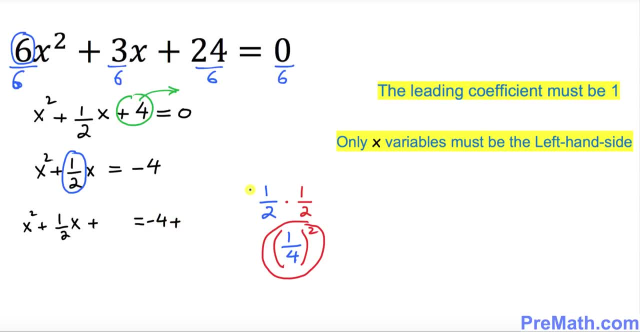 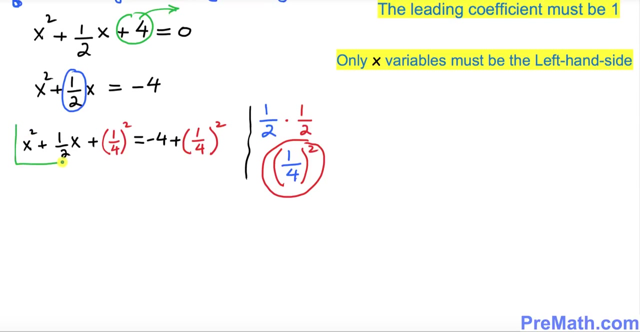 to negative 4 plus Alright. so now we're going to add 1 over 4 squared on this side and 1 over 4 square on this side. As you can see, on the left hand side over here, this represents a complete square of x plus 1 over 4 square, and on this side we can write negative 4. 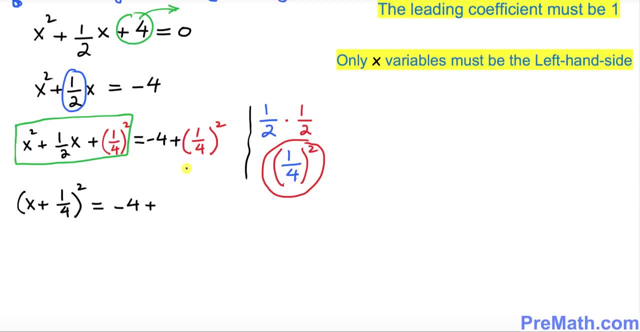 plus 1 over 4 could be written as 1 over 16.. Since we have a fraction over here, we can make this negative 4 fraction by just putting a 1 underneath. If you are wondering, how did we get from this point to this point? how did we get a complete square? we use this well-known fact. 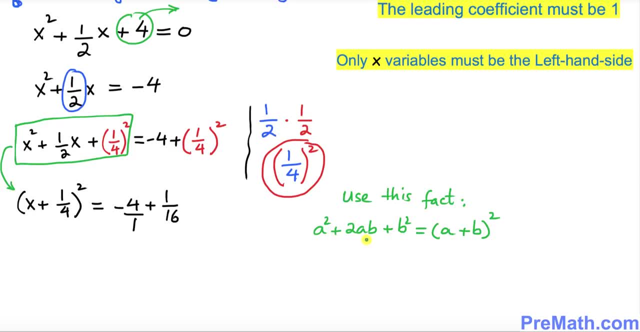 this fact states: a squared plus 2.. 2 times a times b plus b squared is always equal to complete square of a plus b power 2.. So in this case x shows up right here and inside the parentheses, 1 over 4 is right up. 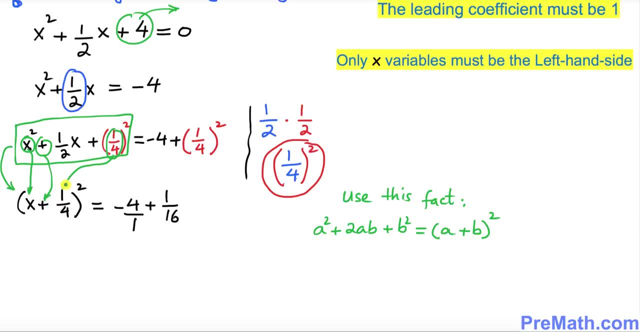 here and this positive sign just got over here. So now we are going to add these two fractions. I put down these two fractions right up here and we are going to simplify adding them by simply cross, multiplying criss-cross. You multiply criss-cross, so that's going to 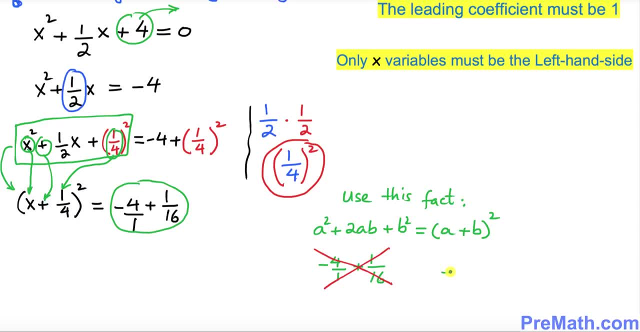 give you. when you multiply negative 4 times 16, that's going to become negative 64, whatever this sign plus, you just put down and then 1 times 1 is 1, divided by your denominators 1 and 16.. You just multiply them out: 1 times 16 is 16, and when you simplify negative 64. 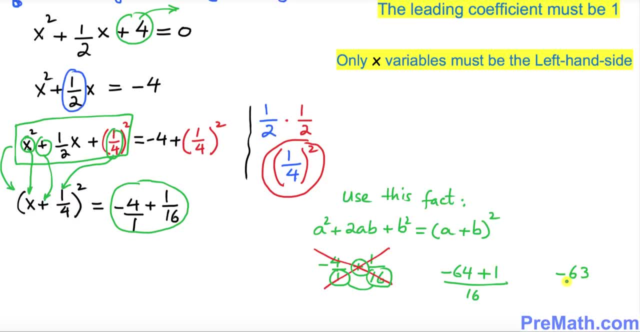 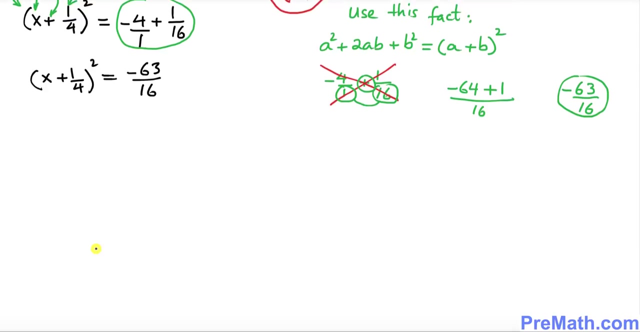 plus 1 is negative 63 divided by 16.. So this is our simplified answer for these two fractions. I just put down negative 63 over 16 and on the left hand side is x plus 1 over 4 square. so far, so good, and now let's go ahead and remove this. 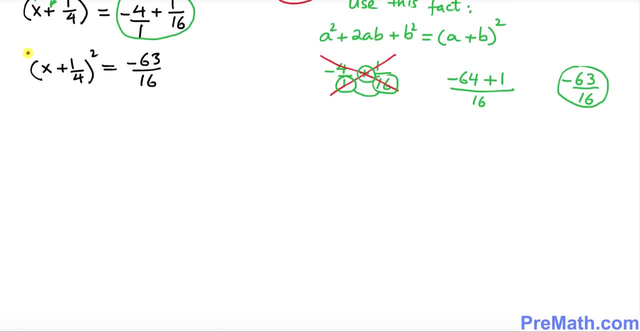 uh, square root, uh, this square. so we're gonna take the square root on both sides, as you can see. so, this square and square root, they undo each other, they cancel each other out. we just simply got x plus 1 over 4 equals to positive or negative, and i can write this thing, i can split it up negative. 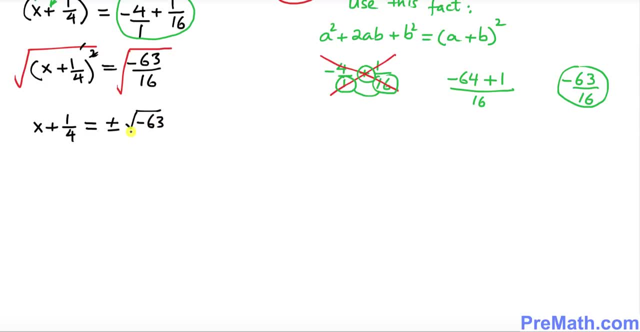 square root of 63 and divided by square root of 16.. and here is square root of negative 63. is could be written as i times square root of 63, where i is an imaginary number and always remember that the square root of negative 1 equals to i. so let's go ahead and simplify this thing so this could be written as: 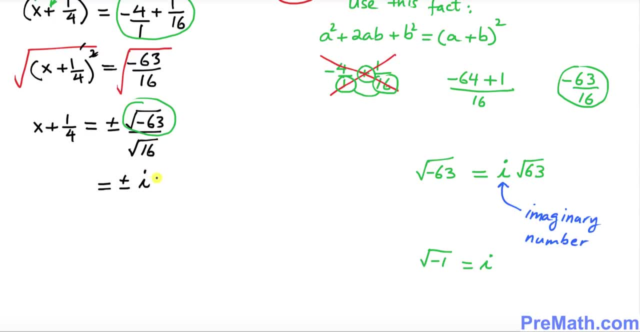 positive or negative. i times: square root of 63 divided by the square root of 16 is 4 and we have x plus 1 over 4.. now we want to isolate x, so we must move this positive 1 over 4 on the other side. so we simply got x equal to this positive 1 over 4 become negative: 1 over 4.